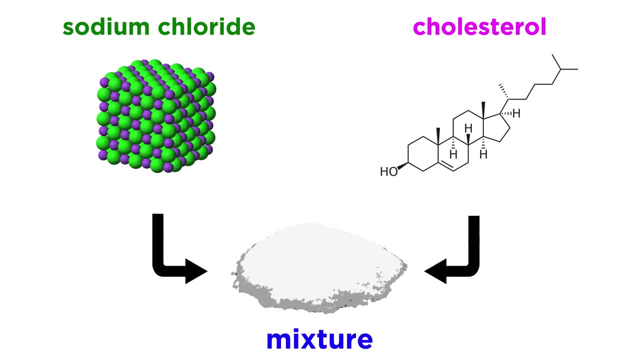 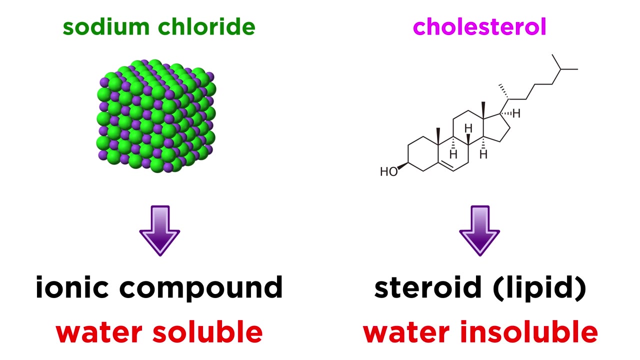 to get them separated again, But in fact, we can use their physical properties to separate them with ease. Sodium chloride is an ionic compound that is water-soluble. Cholesterol, on the other hand, is a steroid, which is a type of lipid and is therefore 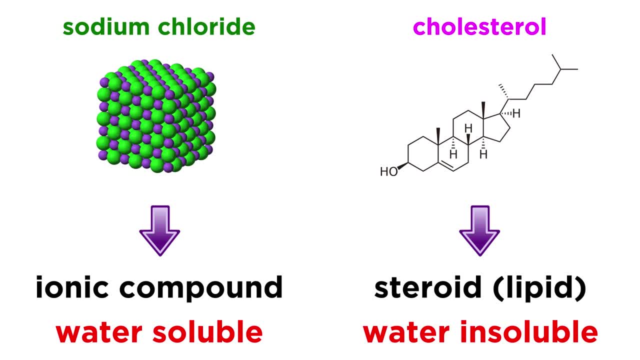 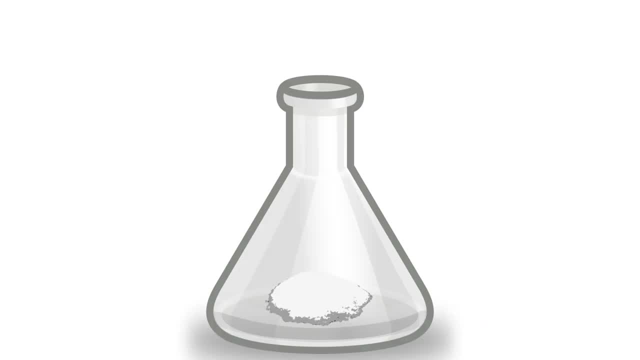 non-polar and largely water-insoluble. However, cholesterol will easily dissolve in a non-soluble solution. Cholesterol is a very important component of the body. It's a non-polar solvent like ether, So to separate this mixture, we would just toss in some water and then some ether. 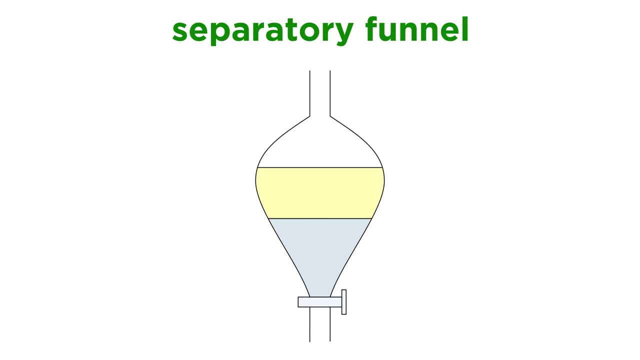 We swirl it around for a while and then put everything in something called a separatory funnel. Since these two solvents are immiscible, meaning they do not mix, we will get two layers. On the bottom will be an aqueous layer which contains all the water and all the sodium. 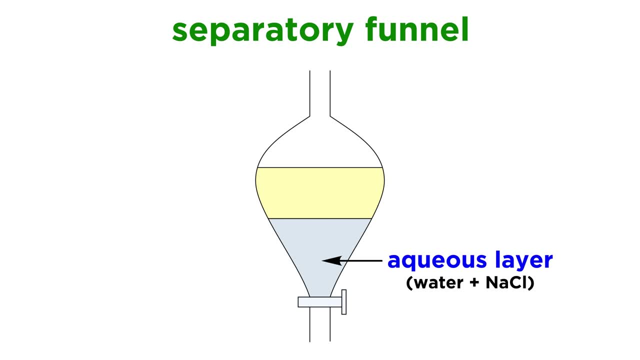 chloride which has dissolved and dissociated. On top will be an organic layer which contains all the ether and all the cholesterol which has dissolved in the ether. The water is on the bottom because it is more dense than the ether, So we just open up the funnel and drain the aqueous layer until we just barely get to. 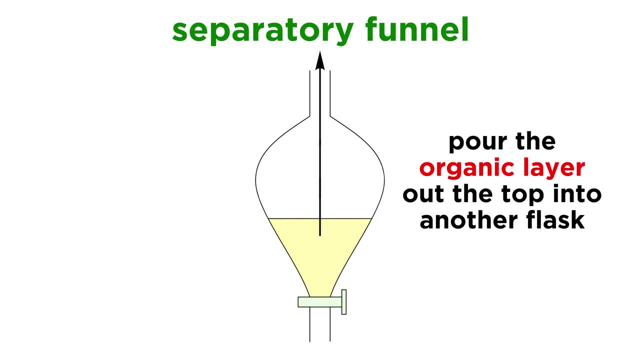 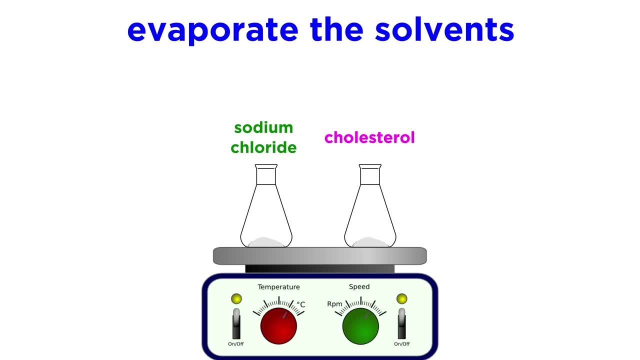 the organic layer And then we pour that out the top of the funnel into something else, Evaporate the solvents And there you have your substances, nice and separated. That one was pretty easy because the substances had differing solubilities. 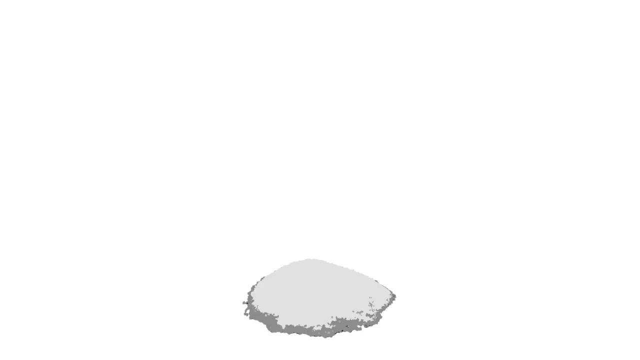 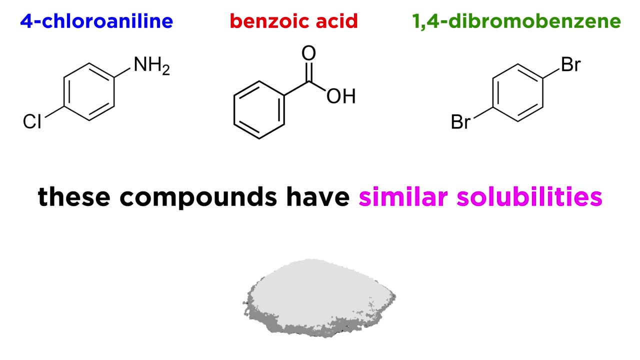 Now let's look at a trickier example. Say we have a solid mixture of four chloroaniline benzoic acid and one four dibromobenzene. These are structurally similar and therefore have very similar solubilities. so we can't 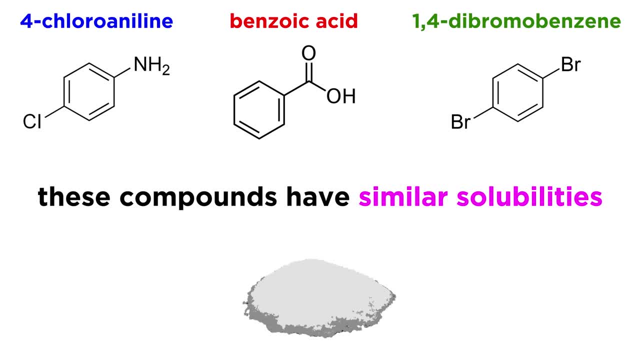 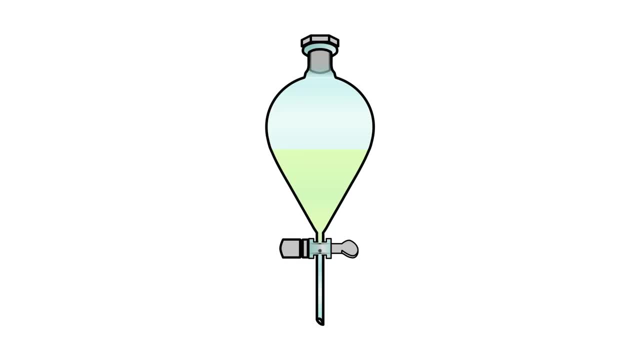 just use two different solvents and expect much to happen. Instead, we have to do some chemistry. Let's toss the mixture in a flask and dissolve it in ether and then transfer over to our separatory funnel. Now let's think: is there some type of reaction that only one of these compounds might undergo? 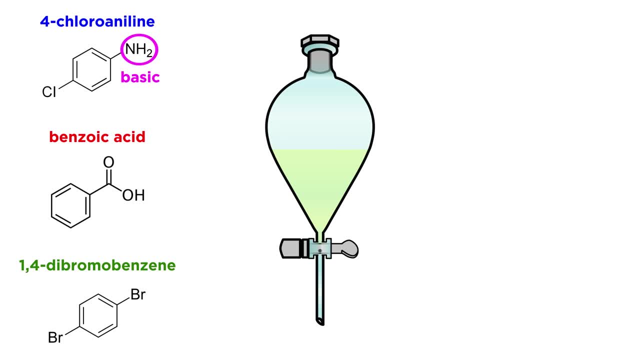 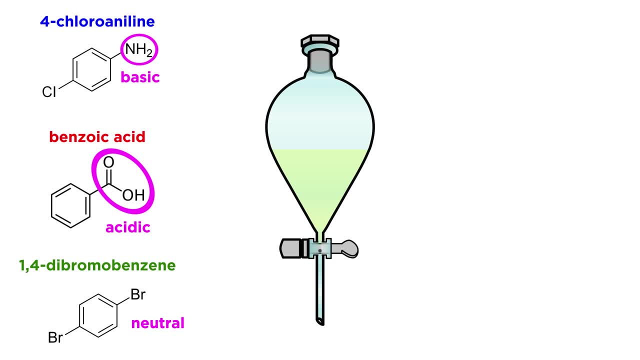 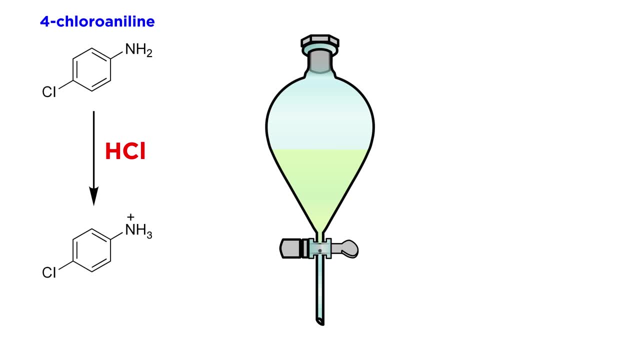 while neither of the other two compounds will react, since they are not at all basic. So let's toss in some of an aqueous HCl solution. Since this is aqueous, it will be more dense than the ether and it will pass right through. 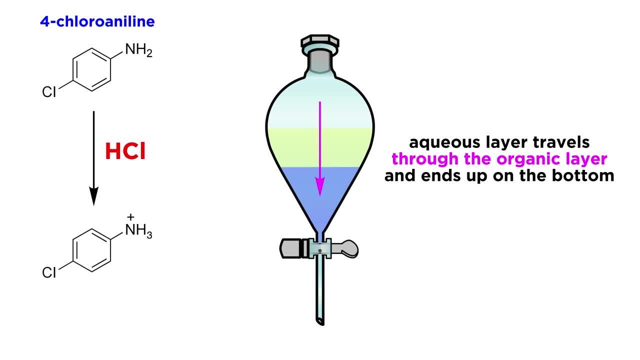 to collect on the bottom, forming an aqueous layer, But as it passes through it will perform acid-base reactions, transferring protons to all the aniline molecules. Once aniline is protonated, the nitrogen atom will bear a formal positive charge. 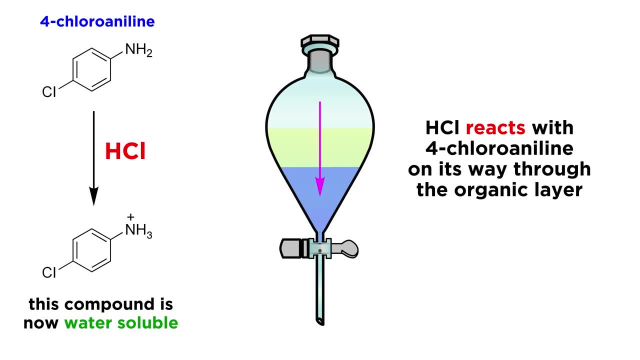 And whereas the neutral aniline was not particularly water-soluble, this aniline salt will be, because the formal charge can make ion-dipole interactions with water that are favorable. So it's as though the acid yanks the aniline. 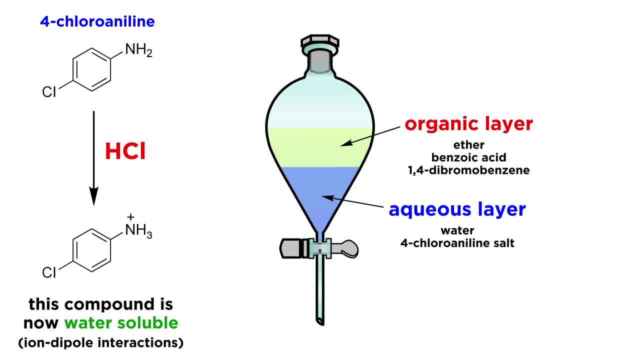 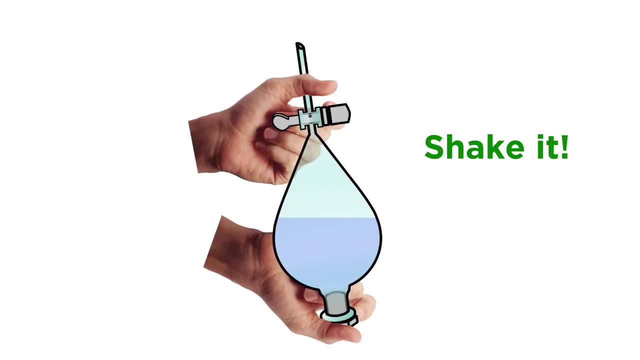 So it's as though the acid yanks the aniline into the aqueous layer as it passes through, Just to make sure everything reacts properly. we will put a stopper over the funnel, pick it up and shake it around a bit. 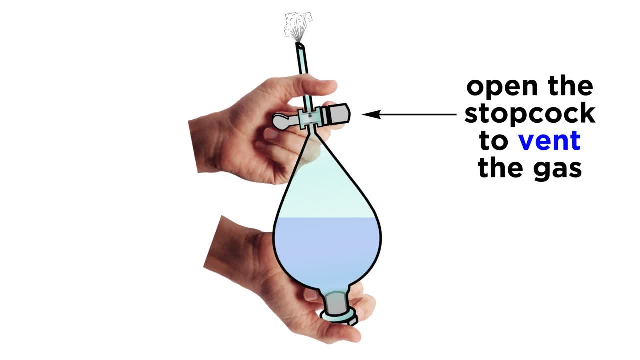 This will generate some pressure inside the funnel, so we will have to periodically vent by holding it upside down with a finger on the stopper and turning the stopcock to release the gas that builds up. This will produce an audible sound. Then close the stopcock and shake some more. 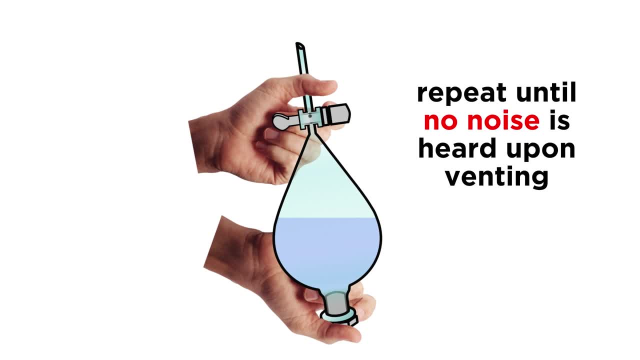 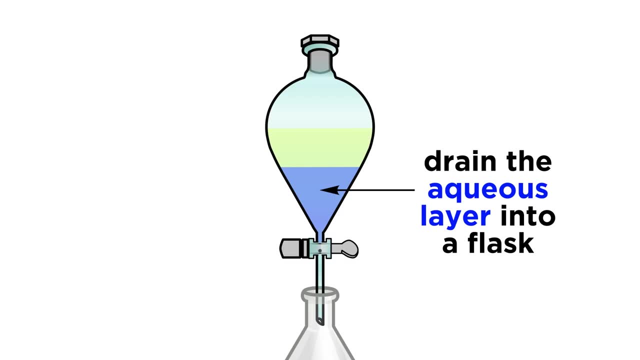 And then vent again. You can keep doing this until the venting doesn't make any more noise. then you know it's done. Then just drain the aqueous layer into a new labeled flask. To be thorough, we will typically wash the organic layer again with another portion of. 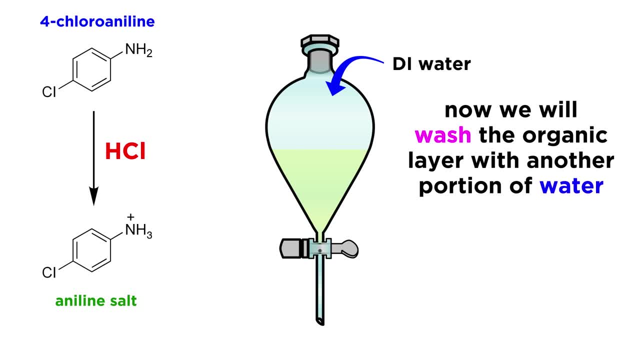 the acid and repeat the whole process and then maybe even one more time with just deionized water, collecting all three aqueous extracts in the same flask. Now we've got our aniline salt sitting in water and we can put it aside for a moment. 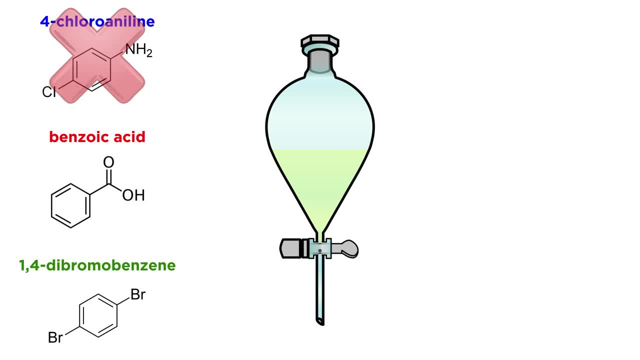 So what's left in the ether? There is benzoic acid and there is dibromobenzene. As you might guess, the next step will be to add some base, since the acid will react while the other compound will not, since it is not remotely acidic. 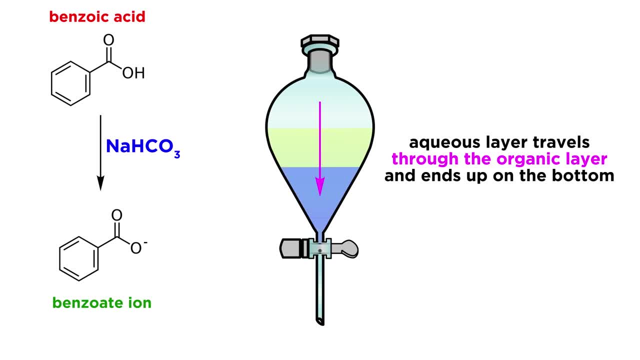 So we can add some aqueous sodium bicarbonate which will pass through the organic layer to form an aqueous layer at the bottom. But as it goes it will accept a proton from benzoic acid. This leaves the benzoate ion, which will be very water-soluble since the negative charge. 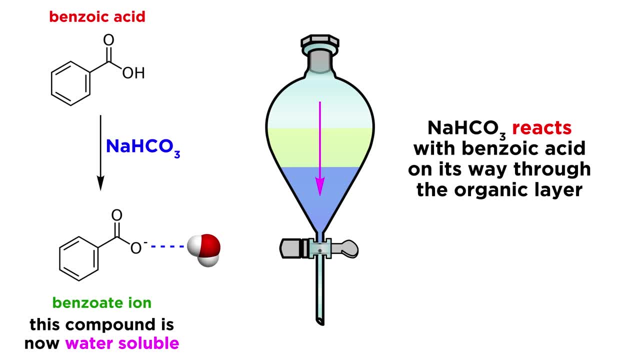 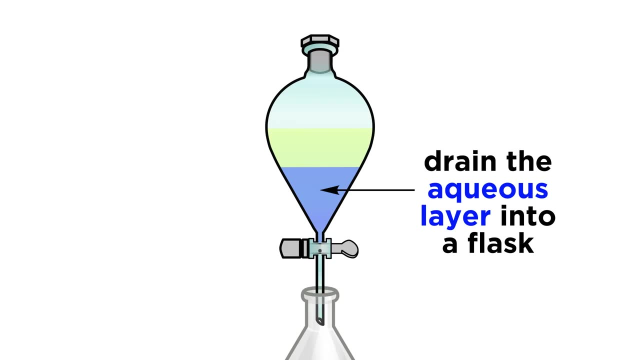 can interact with water molecules in solution. So, just like the previous step, the base drags benzoic acid into the aqueous layer. We perform the same actions as before: shaking, venting, collecting the aqueous layer in another labeled flask. 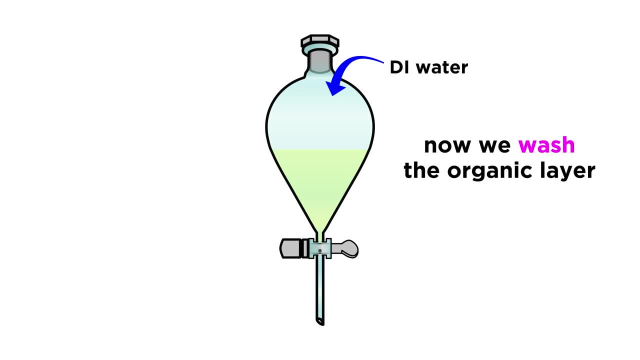 Washing again with base and then again with just water, And now we have our benzoic acid salt sitting in water, which we can put aside. So what's left in the separatory funnel? That will just be the dibromobenzene in ether and we can pour that out the top to avoid. 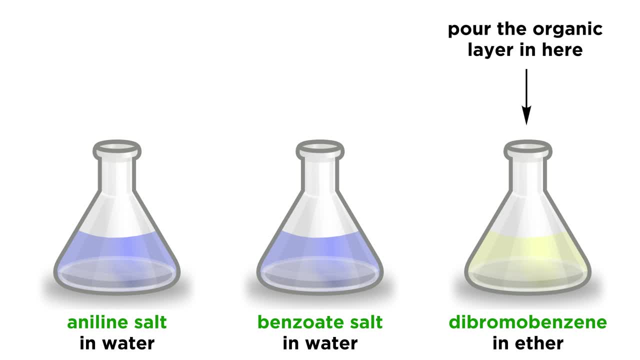 contamination into yet another new labeled flask. Wash the empty funnel with a little ether to make sure we get it all, and add that to the flask. Now toss in a little bit of a drying agent like sodium sulfate to suck up any water. 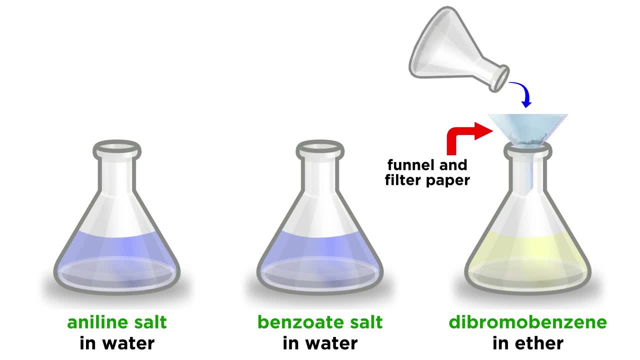 that may have made it in there. Then use a funnel with some filter paper to transfer the solution into yet another flask, this time pre-weighed, if you intend to measure the mass of product. So now we have successfully separated our mixture into its three components. 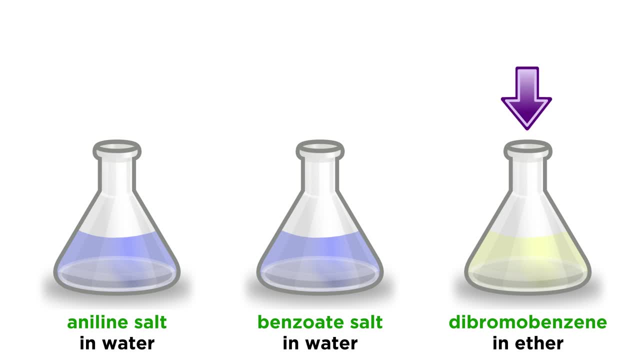 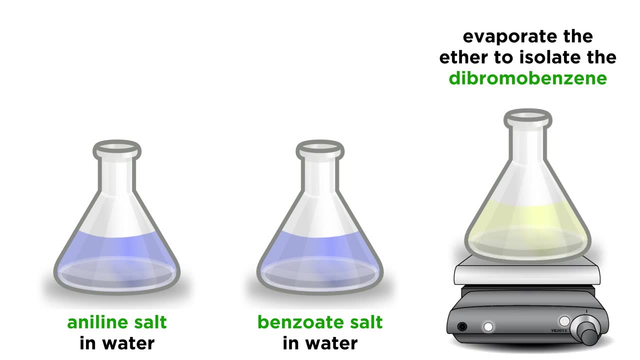 So how do we get the solids back? Well, the dibromobenzene is easy. That's just sitting in ether, and ether is quite volatile, so let's just put it on a hot plate and use a low setting to gently evaporate the ether away. 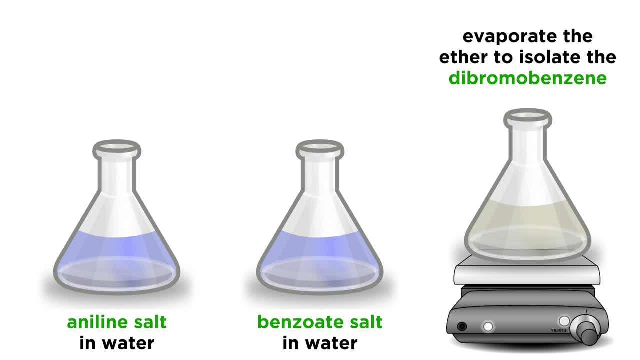 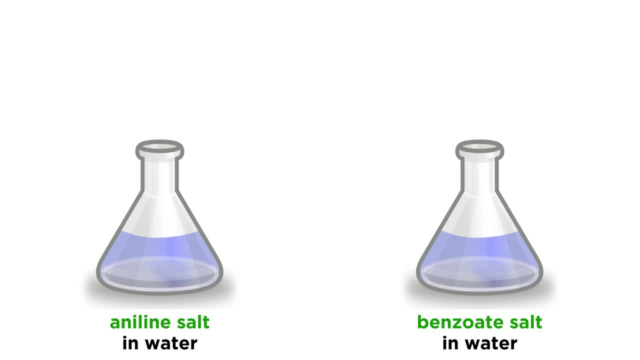 The dibromobenzene will remain as a residue and you can weigh the flask again to get its mass. The other two substances will be a little tricky because they are now salts so we have to do a little more chemistry. The aniline salt needs to be deprotonated, so we need a strong base like sodium hydroxide. 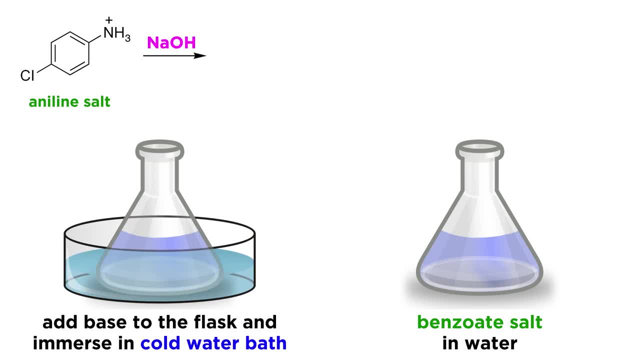 Let's add some of it to the flask, immerse it in a cold water bath and watch the four chloroaniline precipitate. We can be sure that this is finished by checking the pH. Once all the salt has reacted, then no more hydroxide can react and it will thus remain. 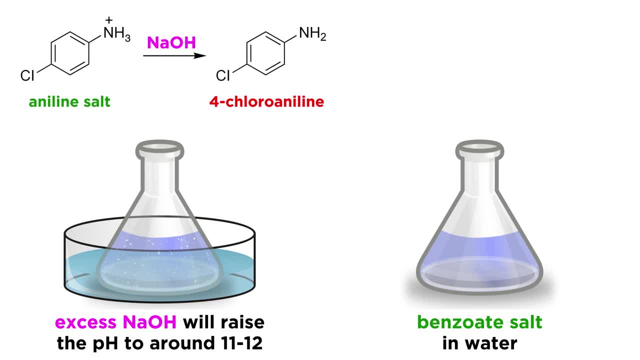 in solution and the pH should reflect that, reaching around 11 or 12.. Now that we have our solids sitting at the bottom, we can just set up a Buchner filter. We can just set up a Buchner filter. Now that we have our solids sitting at the bottom, we can just set up a Buchner filter. 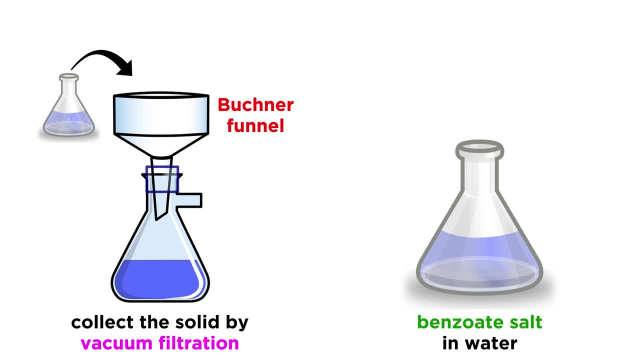 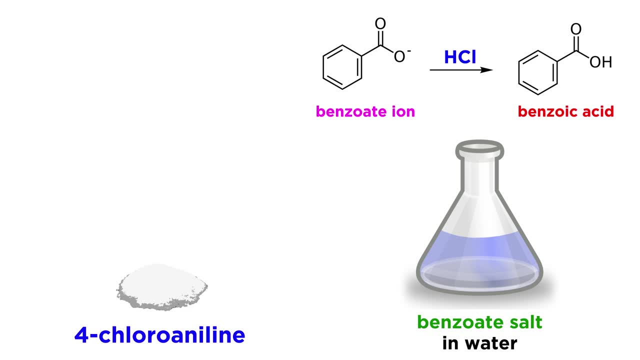 Now that we have our solids sitting at the bottom, we can just set up a Buchner filter. We can just set up a Buchner funnel, hook it up to a vacuum pump, pour the solution onto the filter paper sitting in the funnel and wait for it to dry. 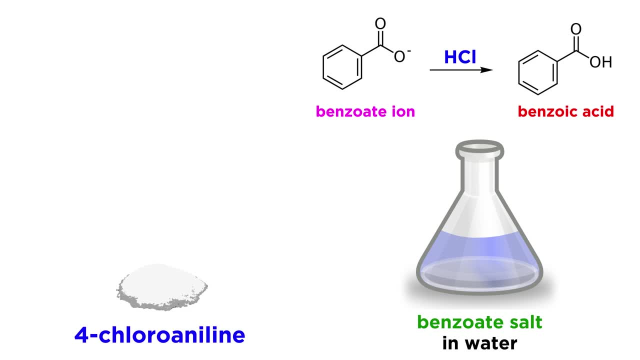 Then we can do the same thing with the benzoic acid salt, except here we need a strong acid to protonate it. So to this flask let's add some HCl. watch benzoic acid precipitate. check for a pH. 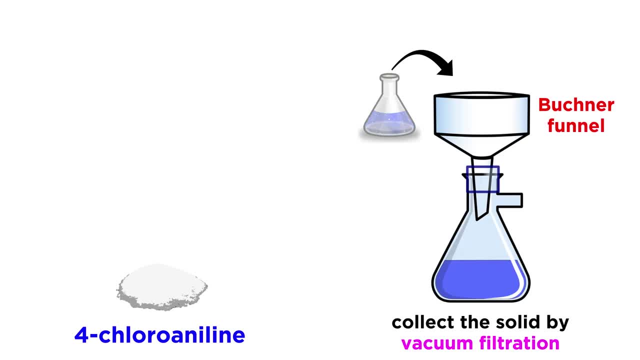 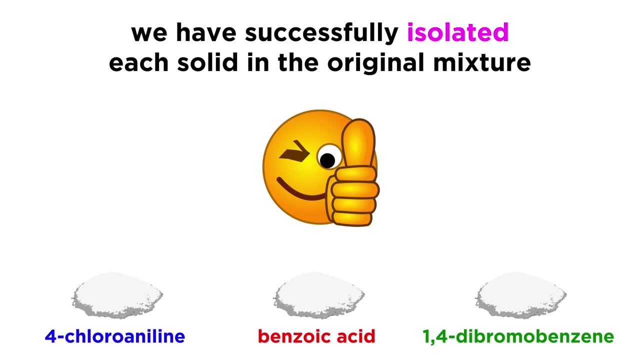 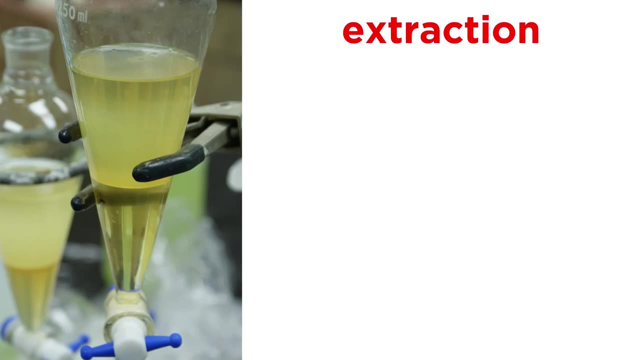 of around 2 to ensure that this is complete, and then collect that in a Buchner funnel as well, And there you have your three solids completely separated. So hopefully we now understand what extraction is and how it is performed. This technique is ubiquitous in the organic chemistry laboratory. 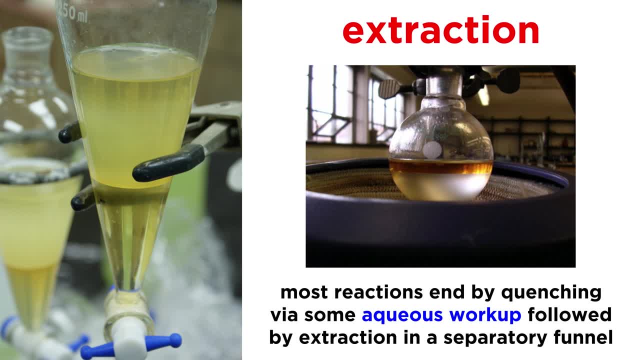 Almost every single time a reaction is performed, it will end with some kind of aqueous workup to neutralize any ionic products, after which the contents of the reaction flask will be transferred to a separatory funnel for extraction. So if you are interested in doing a lot of organic chemistry, make good friends with 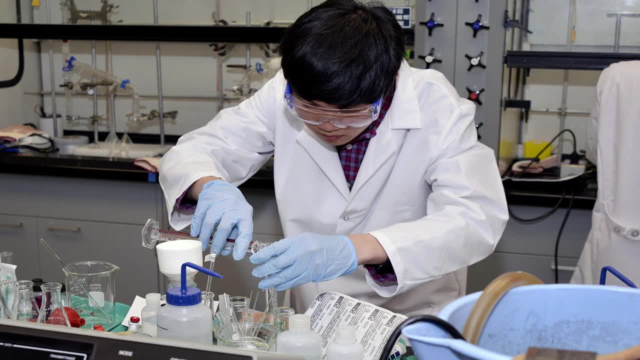 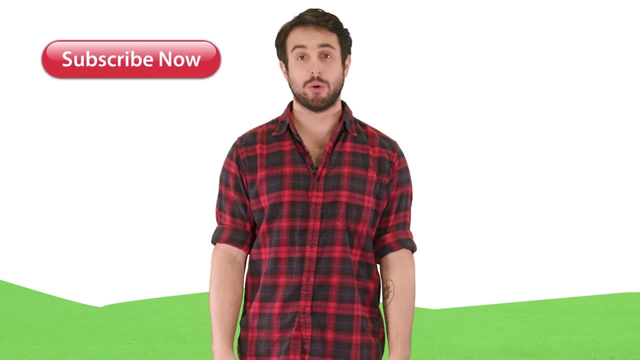 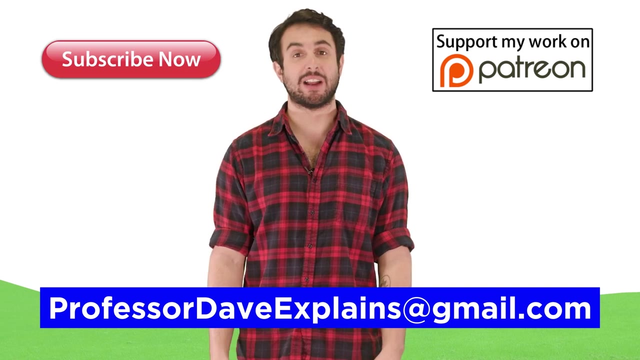 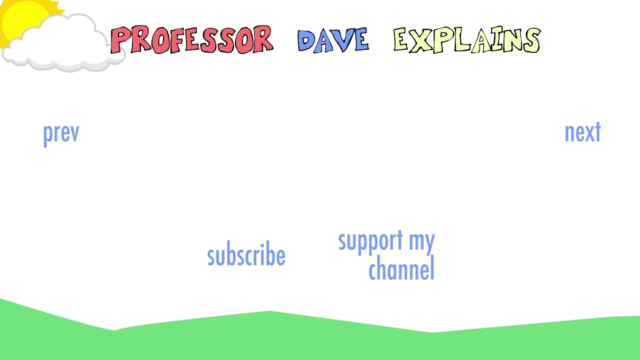 your separatory funnel now And with this technique understood, let's move forward and learn about some others. Thank you very much for watching and I'll see you in the next video.